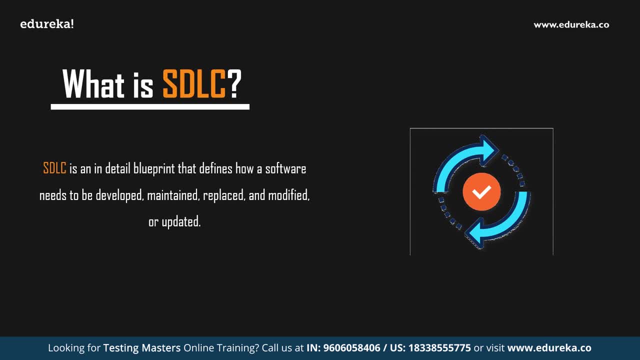 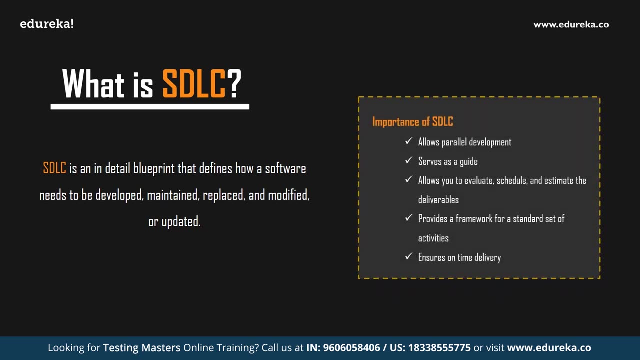 maintained, replaced and modified or updated the software development life cycle. It outlines a methodology for the betterment of the software quality and the overall development process. the importance of software development life cycle: as I've mentioned earlier, software development is a very long process and therefore it requires to be carefully planned and executed. 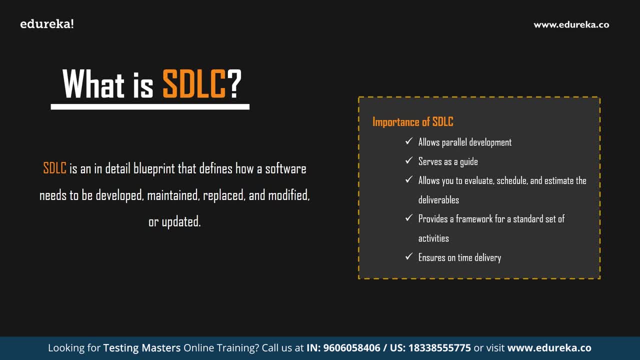 So this is where SDLC comes into focus. the software development life cycle breaks down the entire process of software development, thereby making it easy to understand and evaluate each and every part of the software development process. Not just that, SDLC also provides other benefits, such as allowing the software development team 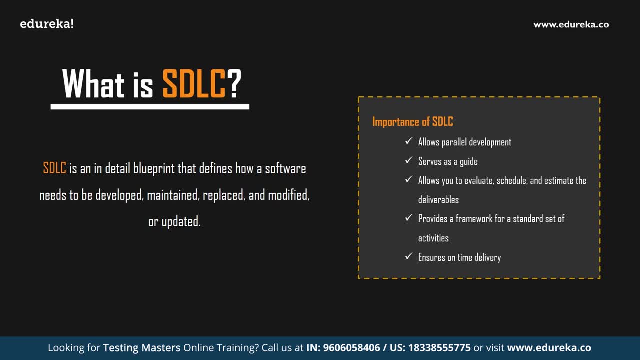 to work parallelly on each phase. It serves as a guide for the software under development and helps meet the clients requirements. SDLC allows us to evaluate, schedule and estimate the deliverables. It also provides a framework for standard set of activities and ensures on time software development and delivery. 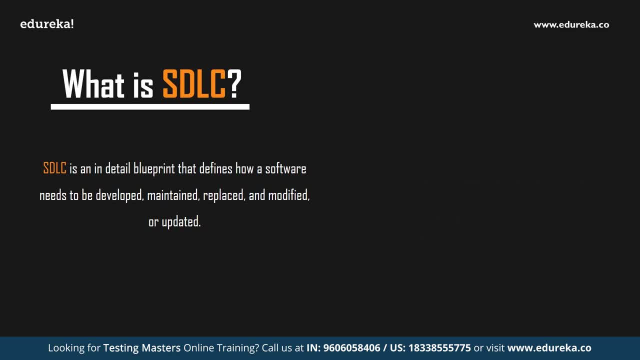 So, moving on towards the phases of SDLC, SDLC, or the software development life cycle, consists of seven phases. I'm not going to discuss these phases in detail over here, because we're going to take a look at them when we're comparing SDLC and SDLC. 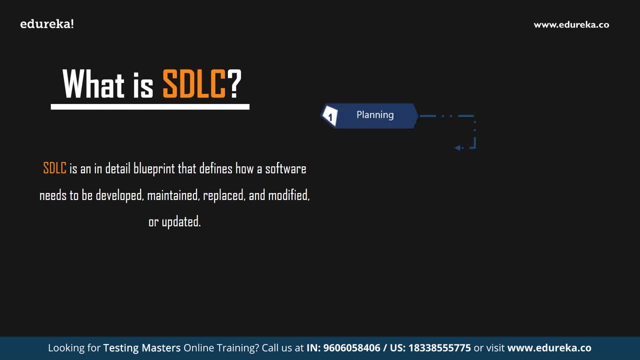 the phases that are present in SDLC are the planning phase, which highlights what software is to be developed. deployment analysis phase, wherein a team of Engineers perform a feasibility study of the software that is under consideration And jot down all its requirements. then is the designing phase. 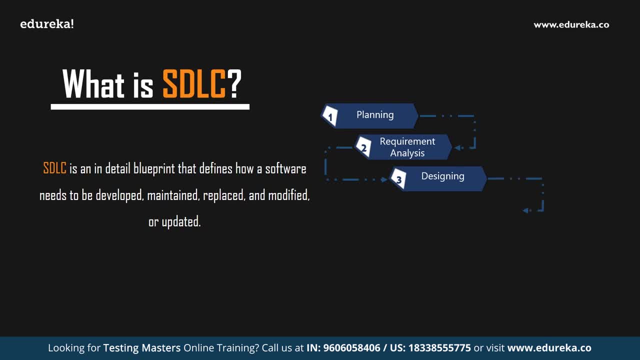 the design phase, as the name suggests, is a phase wherein technical Architects provide high-level and low-level design to the software that is under development. Next up is the implementation, or the coding phase. Once the coding is completed, the software then is tested in the testing phase and then deployed in the deployment phase. 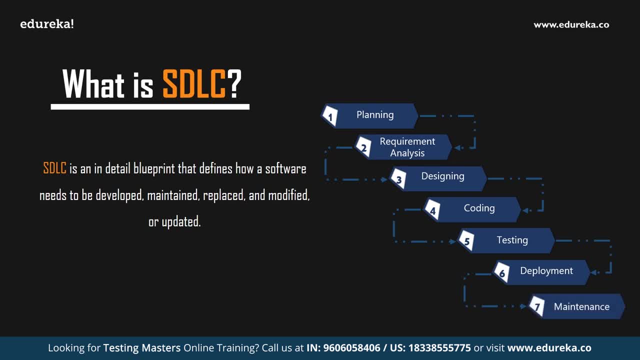 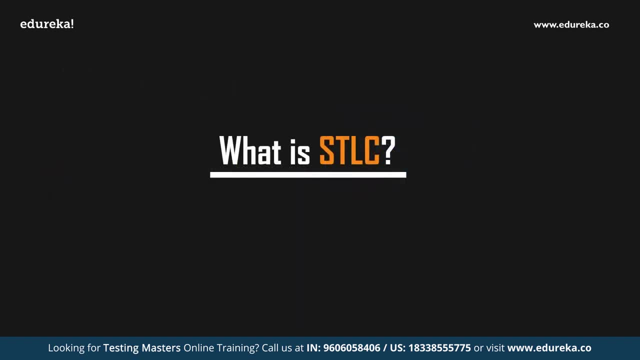 Finally, once the software is into production, it has to be maintained and updated, which takes place In the maintenance phase. So those were the phases of SDLC. Now let's move on and understand what exactly is SDLC. SDLC stands for software testing life cycle. 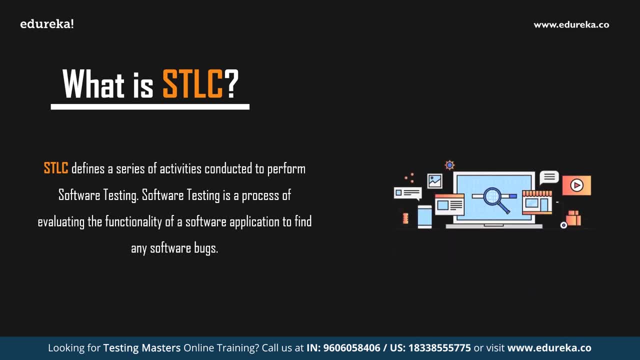 It defines a series of activities conducted to perform software testing. software testing is a process of evaluating the functionality of a software application to find any software bugs. It checks whether the developed software met the specific requirements and identifies any defect in the software in order to produce a quality product. 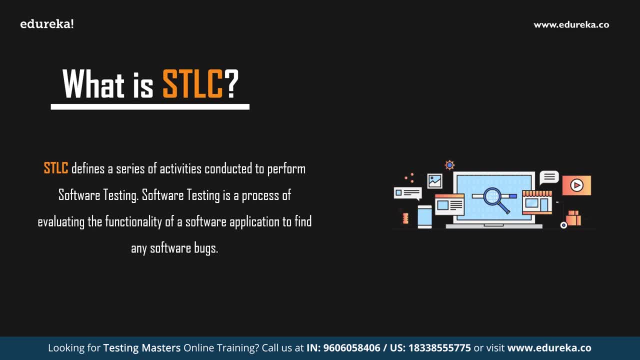 It is also stated as a process of verifying and validating a software product. Therefore, it basically checks whether the software product that is developed meets the business and the technical requirements that guided its design and development, if it works as per the requirements and can it be implemented with the same characteristics. 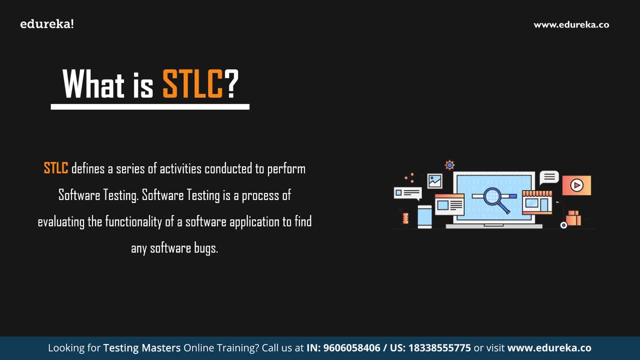 SDLC identifies what test activities to carry out and when to accomplish these test activities. In the SDLC process, Each activity is carried out in a planned and systematic way, and each phase has different goals and deliverables. So why is testing important? software testing is important. 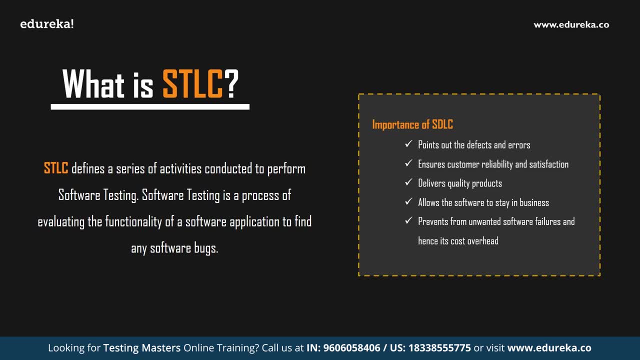 because of the following reasons: it points out the defects and errors that were made during the development phases. It looks for any mistake made by the programmer during the implementation phase of the software. It ensures that the customer or the client finds the organization reliable and their satisfaction. 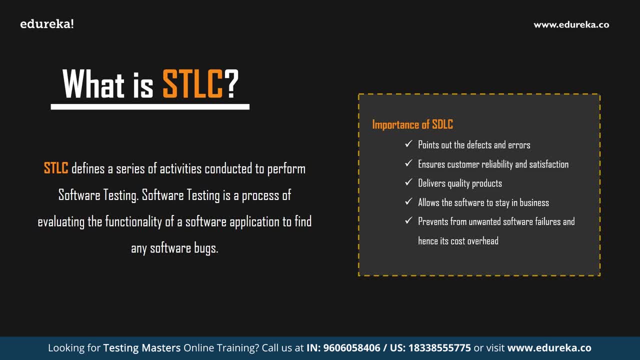 In the application is maintained. sometimes, contracts include monetary penalties with respect to timeline and quality of the product, and with software testing these monetary losses can be prevented. software testing also ensures the quality of the product. the quality of the product delivered to the customers helps in gaining their confidence. 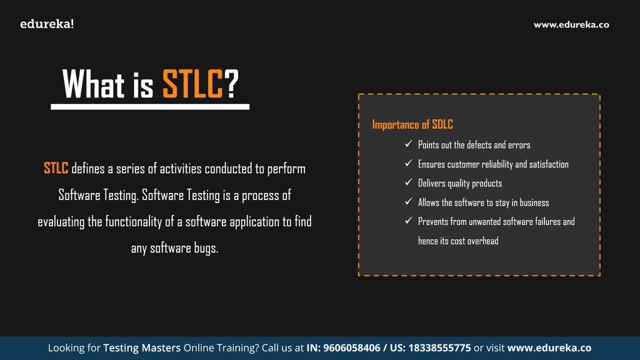 It makes sure that the software application requires lower maintenance costs and results in more accurate, consistent and reliable results. users are not Inclined to use software that has bugs. They may not adopt software if they are not happy with the stability of the application. testing is important for the product to stay. 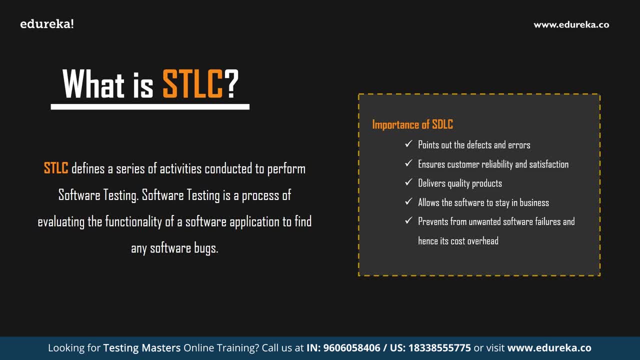 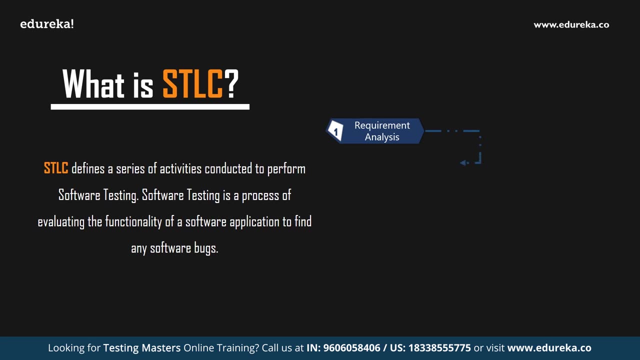 in business. It is also very important to ensure that the application should not result in any failures, because it can be very expensive in the future or in later stages of development. So the phases that are present in software testing are the requirement analysis phase, which is very much similar to the software development. 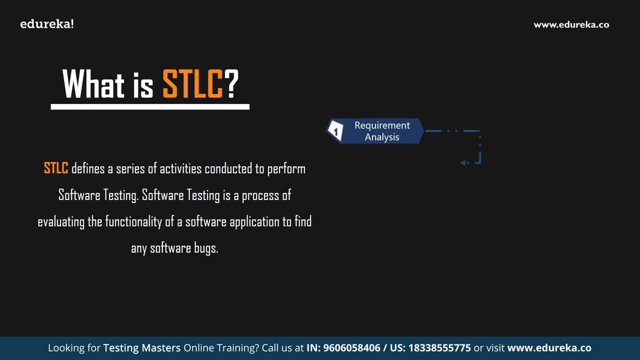 lifecycle phase. But over here, all the requirements that are necessary for testing are penned down. next up is the test planning phase, followed by test case development, environment setup, test execution and, finally, test cycle closure. So now that you are aware of both SDLC and SDLC, including their 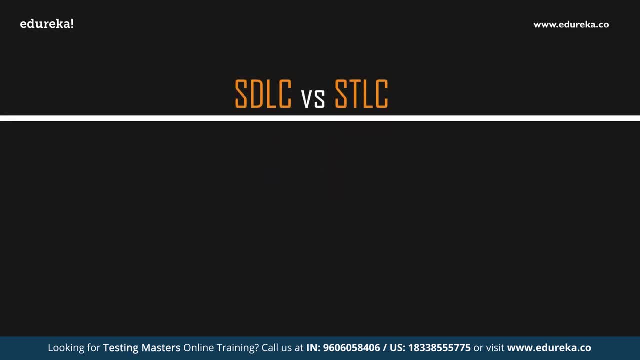 importance and phases. let's move on and compare them with each other. So the first comparison factor that we'll be considering over here is the origin. software development lifecycle begins With the development of the software, since it deals with the development of the software itself, SDLC, or software testing. 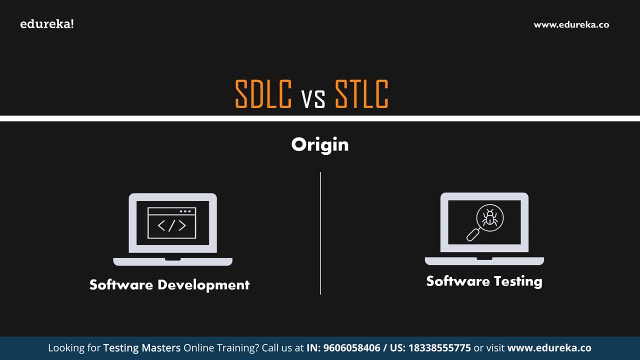 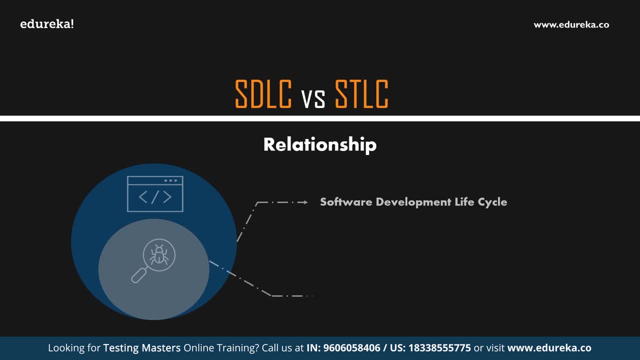 lifecycle, On the other hand, begins when the software is to be tested. the relationship, software development lifecycle can be considered as the parent of the software testing lifecycle. This is because testing is a part of software development. In other words, SDLC can be considered as a child of SDLC. the intention: 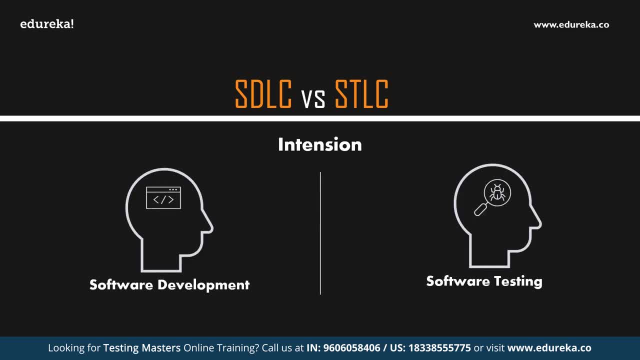 the main reason To formulate a software development lifecycle is to be able to develop quality software smoothly. without SDLC, There are chances of losing track, leading towards no or undesired results. SDLC, or the software testing lifecycle, is formulated so as to detect, analyze and debug any errors or shortcomings of the 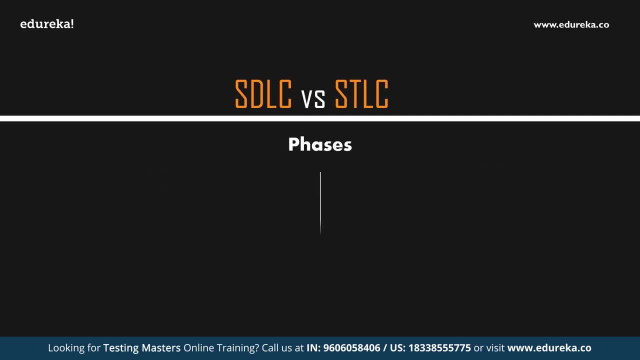 software that is being developed. the phases, as mentioned earlier, the phases that are present in SDLC are the planning phase, requirement analysis phase, design phase, implementation or the coding phase, testing phase, deployment phase and the maintenance phase. on the other hand, the testing lifecycle consists of phases such as requirement analysis, 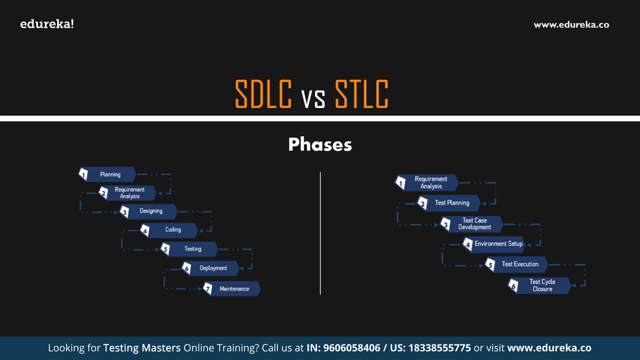 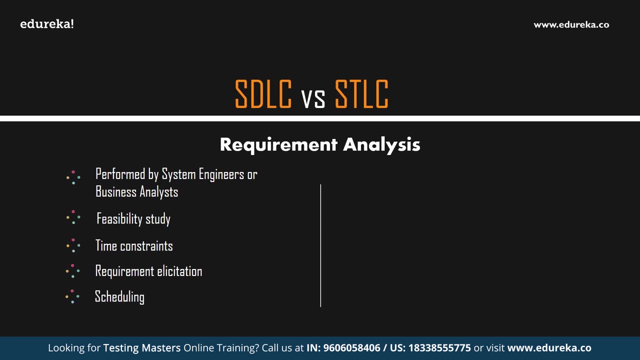 test planning, test case development, environment setup, test execution and test cycle closure. the requirement analysis phase. requirement analysis in SDLC is carried out by a team of software engineers or business analysts, Depending on the Organizations. they perform the feasibility study of the software that is under consideration, the time required to develop the software, the. 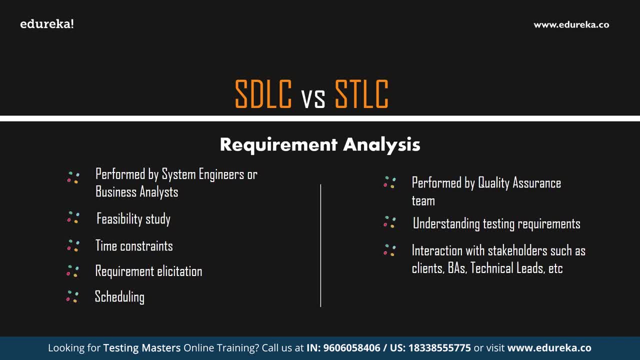 cost, overhead requirement, elicitation, scheduling, Etc. The main focus is to do a final check before the development actually starts. any shortcomings discovered will be sorted out with the development team and stakeholders in SDLC or the software testing lifecycle. This step is carried out by the quality assurance team or the quality 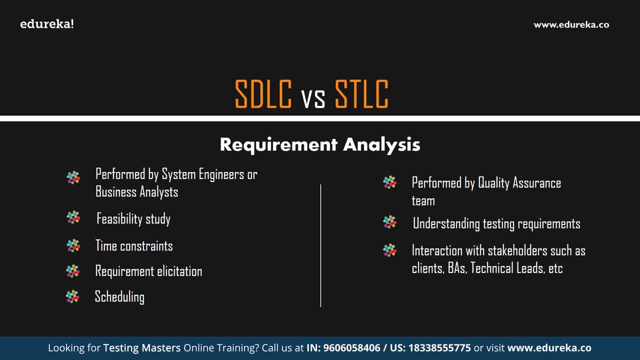 analysts. They understand the requirement in terms of what they will be testing and figure out the testable requirements. during this phase, the test team studies the requirements from the testing point of view. to identify the testable requirements, the QA team may interact with various stakeholders, such as the clients, business analysts, technical leads, system architects. 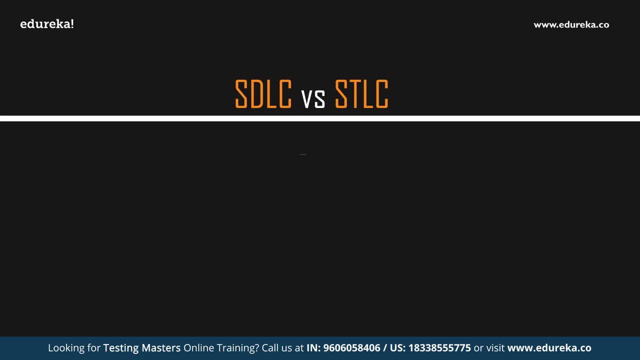 Etc, So as to understand the requirements in detail. the design phase, the design phase in SDLC, is carried out By developers and technical Architects, who start the high-level and low-level designing of the software that is under development. the design phase is formulated in such a way that it delivers each 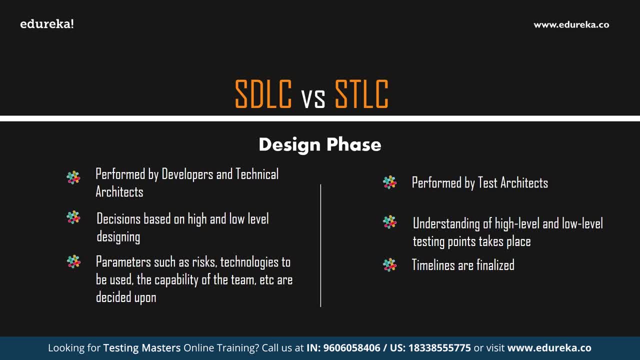 and every requirement that is specified. during the requirement analysis phase, all the technical details of the design are discussed with the stakeholders and various parameters, such as risks, technologies that are to be used, the capability of the team, project constraints, time and budget, are reviewed, and then the best design. 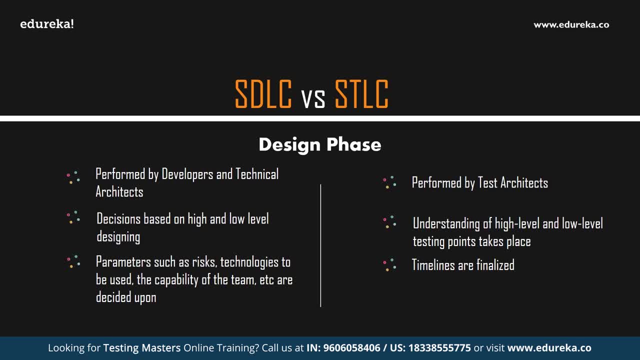 Approach is selected for that product. in software testing lifecycle test Architects are the ones who govern the activities, do the test planning and identify high-level testing points. All the resource allocations and timelines are also finalized in this phase, the coding phase. in the coding phase of SDLC, the design of the 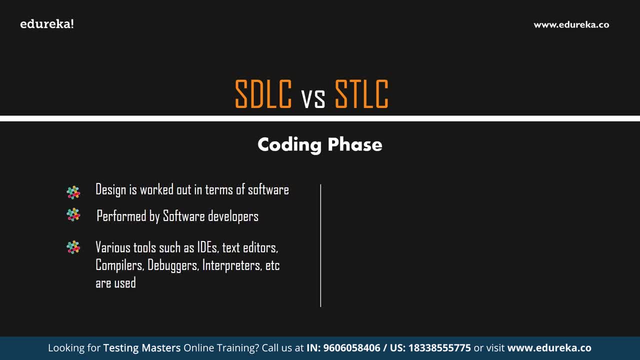 software is worked out as a piece of software. software developers play a prominent role in this phase. It includes various details, Such as the programming language that is to be used, the best fitting framework, the most suitable methods. Etc Developers make use of various programming tools, such as IDs text. 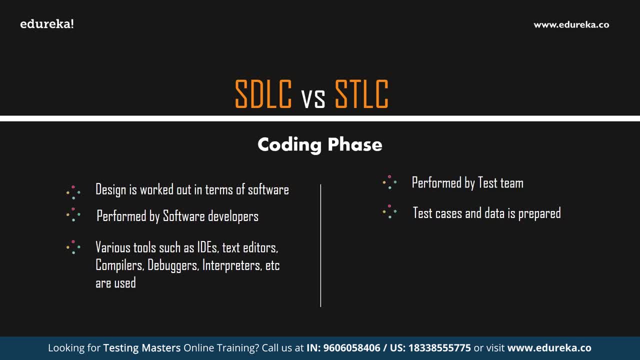 editors, compilers, debuggers, interpreters, Etc. This is the longest phase of the software development lifecycle. The test case development begins once the test planning phase is completed. This is the face of SDLC, where the testing team notes the detailed test cases Along with test. 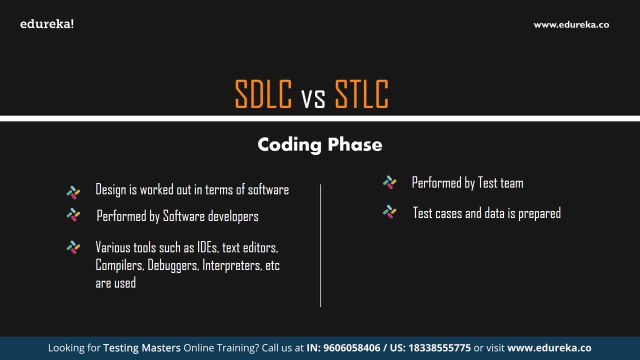 Cases. the testing team also prepares the test data for testing. once the test cases are ready, They're then reviewed by the peer members or the QA leads. a good test case is the one that is effective at finding defects and also covers most of the scenarios on the system under test. 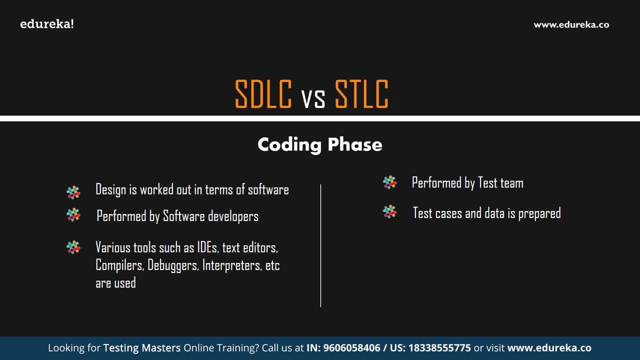 Let me just list down a step-by-step guide on how to develop a good test case. Remember that the test cases need to be simple and transparent. create a test case with the end user in mind. Avoid repeating the test cases over and over again. do not assume the 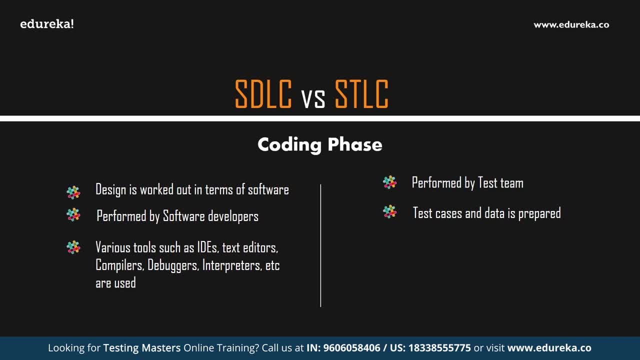 functionality and features of your software application. ensure hundred percent coverage of the software requirements. name the test case ID such that they are identified easily while tracking defects. implement the testing techniques. the test case you create must return test environments to the pretest state. The test case should generate the same results every time. last but not, 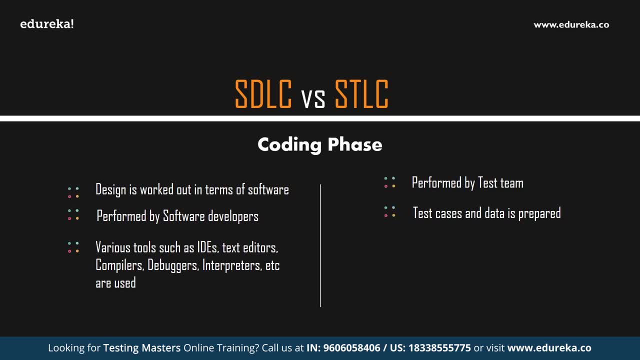 the least, Your peers should be able to uncover defects in your test case design as well. So, moving on towards the final comparison factor, which is the testing phase, in SDLC, the actual testing of the software is carried out in the testing phase. It can be done using any of the testing methods, such as unit testing. 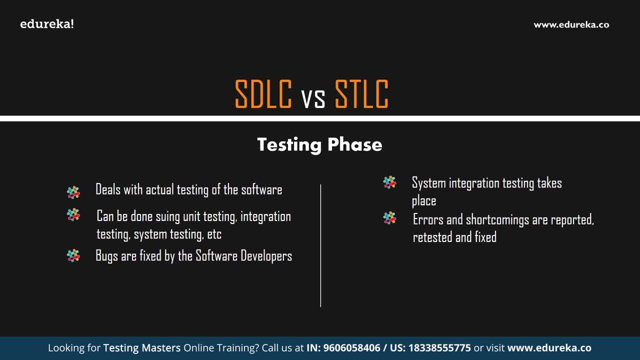 integration testing, system testing, defect resisting, regression testing, Etc. All the bugs that are reported are then fixed by the software development team. Once the errors have been sorted, the software is sent back to the tester so as to recheck the software in SDLC system integration testing. 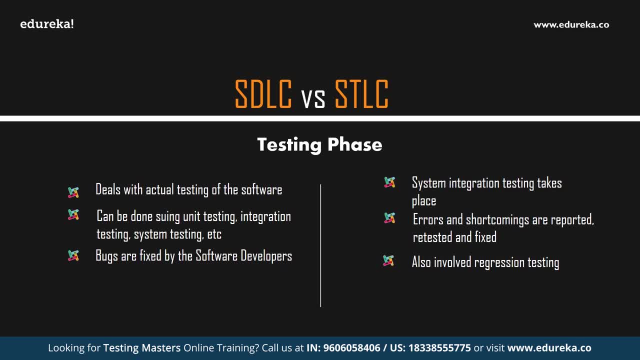 takes place based on the test cases. all errors and shortcomings that are reported get to retested and fixed. this team also performs regression testing and the software is signed off once it means the exit criteria. Okay, So, as we've seen, SDLC and SDLC might have a similar name but are quite 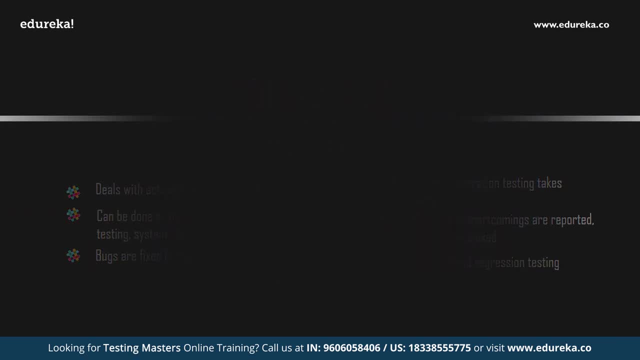 different when it comes to their functionalities. This brings us to the end of the session. I hope you guys have enjoyed and learn something new. in case you have any doubts or queries, please do let me know in the comment section and I will revert to you at the earliest. 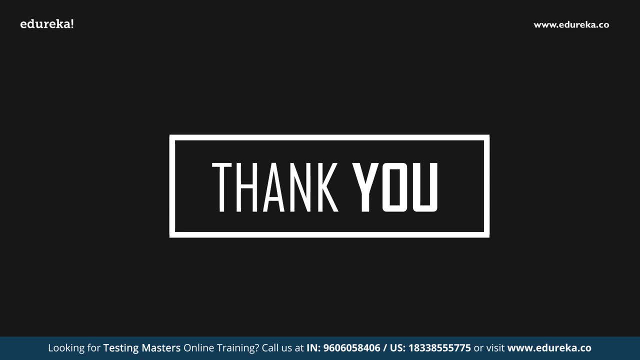 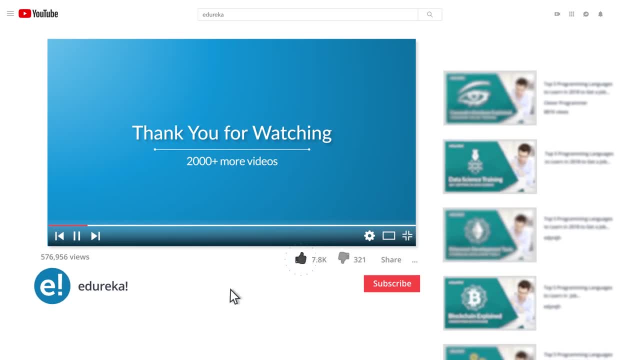 We'll be back with more and more exciting sessions, but still then, goodbye and take care. I hope you have enjoyed listening to this video. Please be kind enough to like it and you can comment any of your doubts and queries and we will reply them at the earliest. 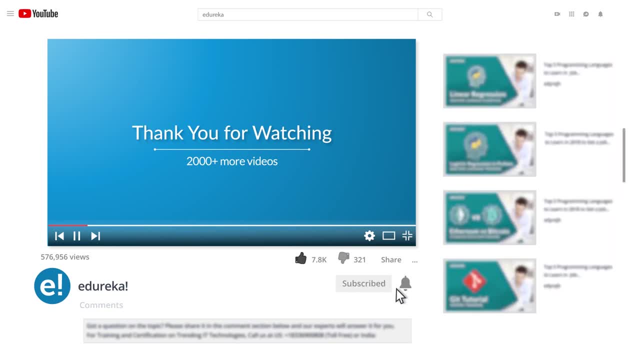 Do look out for more videos in our playlist and subscribe to edureka channel to learn more Happy learning.